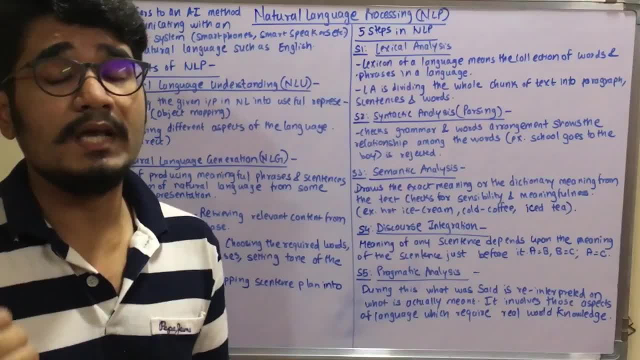 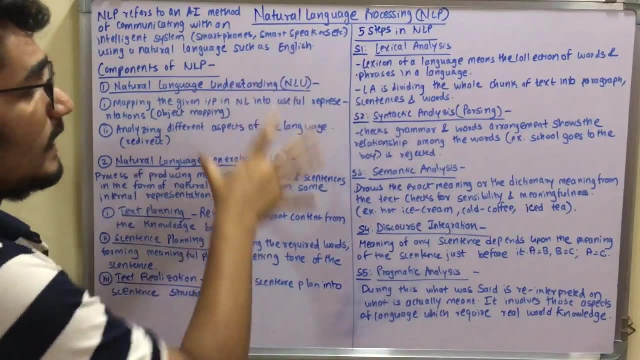 turn your music system on. they will turn your lights on fan on, and not what? not everything they will on by themselves. so by using all natural language, such as english. so english is the base language for all these things in order to command like you have, if you are. 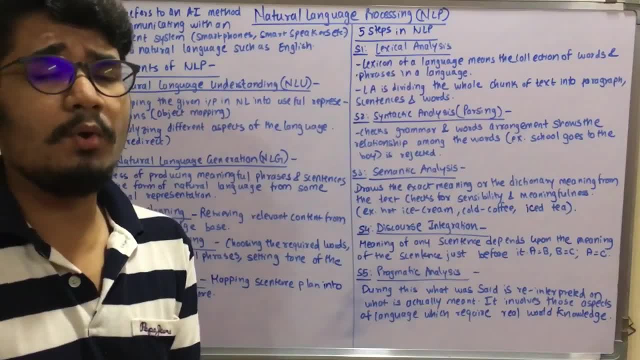 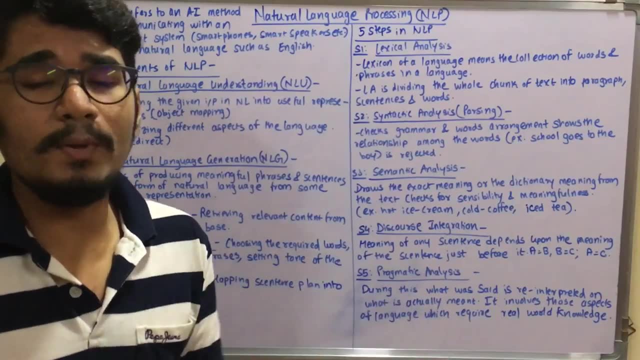 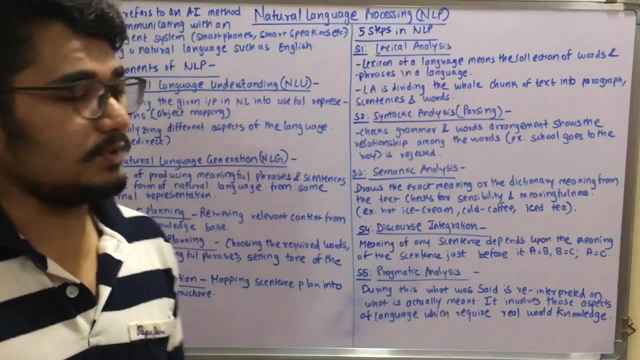 having german language, spanish, russian and all these things, then you have to manually code and sit and make those system design to understand what these things actually mean, and so english is our natural or global language. it becomes very easy for us to communicate and also for machines to communicate in a global fashion, and so there are two components. 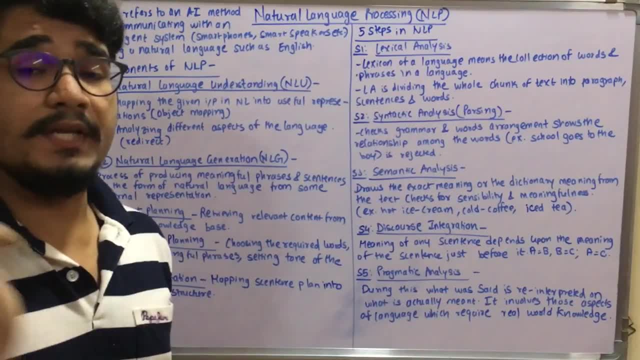 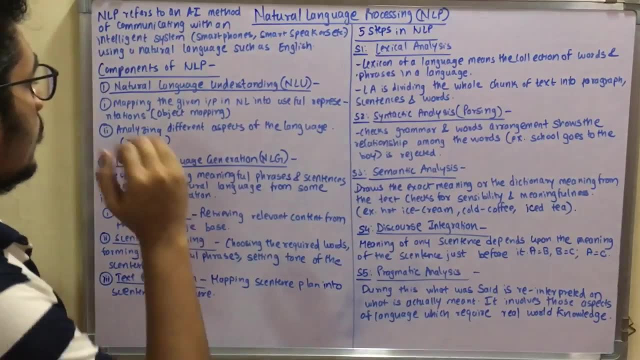 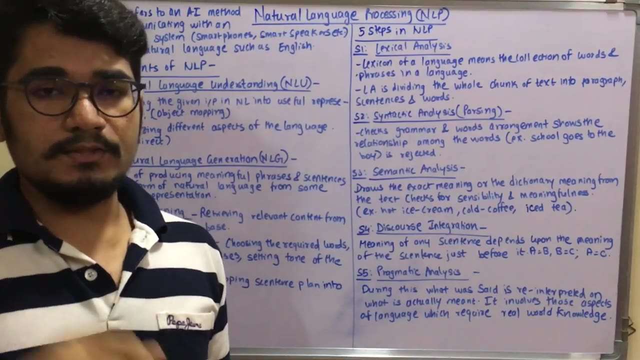 two major components contributing to nlp. that is, we have the very basic components, which are: the first one, that is, natural language understanding, and then you have the natural language generation. so let's go one by one. so what is natural language understanding? you have to understand the natural language, like, for example, say, a baby, is there a small? 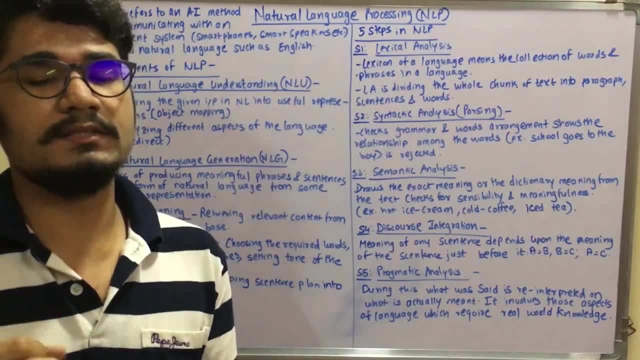 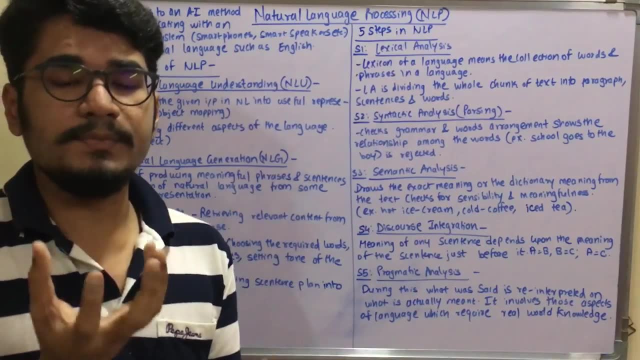 kid is there now. he wants to understand an english language. so what he does is he studies a for apple, b for ball, c for cat and all these things. so he has to get those objects from the real world and he has to just visualize these things are called in that way, that's. 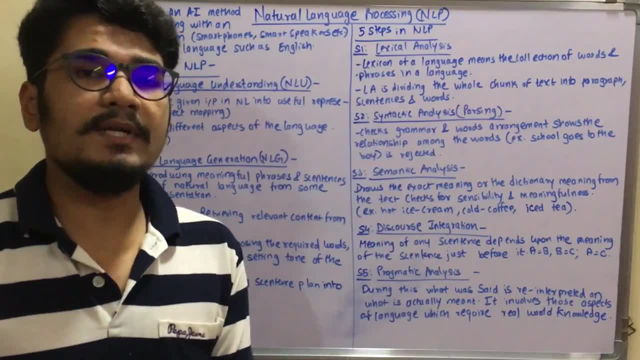 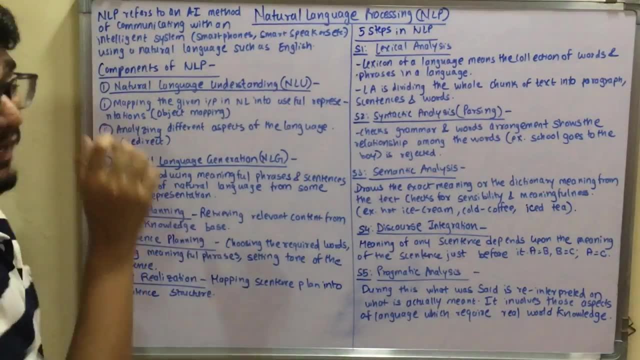 why the c for car is there, c for cat is there, a for apple is there and a for aeroplane, b for ball and so many things. so it has to get that object in his hand. so the very first goes in natural language. understanding is mapping of the given input in natural language. 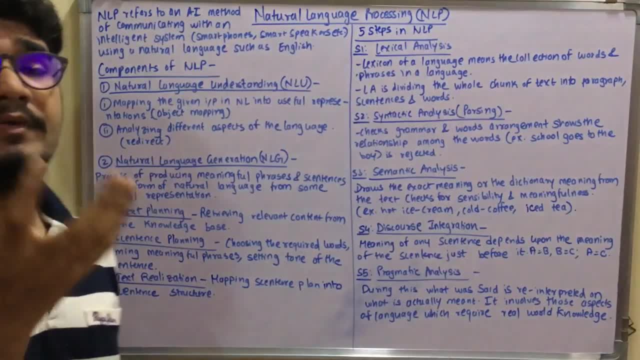 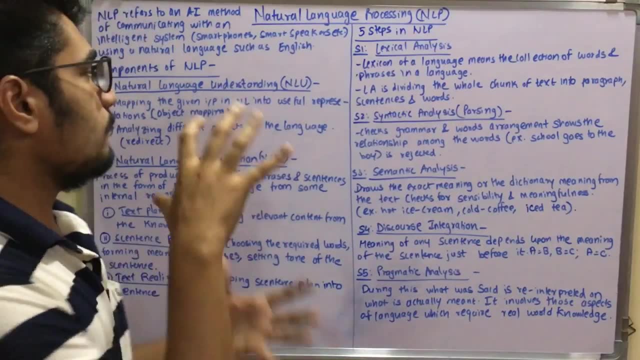 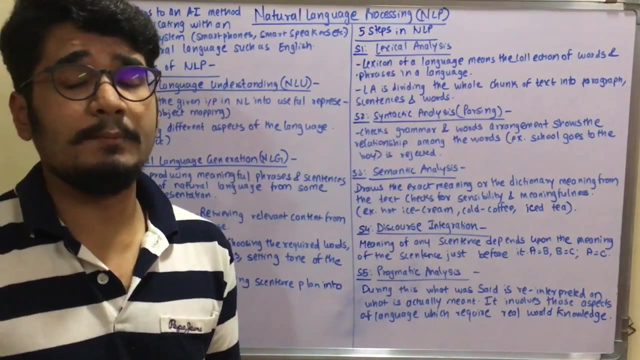 into useful representations, like we have the object mapping. you have different objects in the real world, so from that you just map those into different, different forms in your understandable things. so the very challenging thing in nlp that i would say is you have to understand the kind of language. so it's very difficult, like tomorrow if i'm learning. 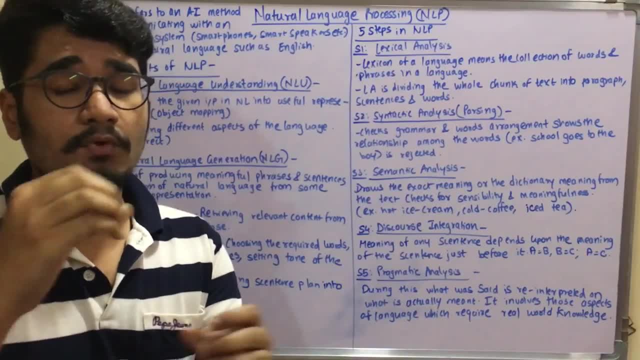 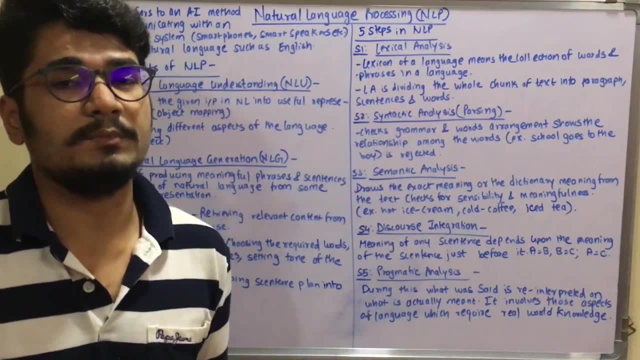 german language. then it becomes a challenge for me to understand what and everything is called, like a pen is called what in german, a book is called what in german or in a house is called what in german. so all these things i have to get those things means i should. 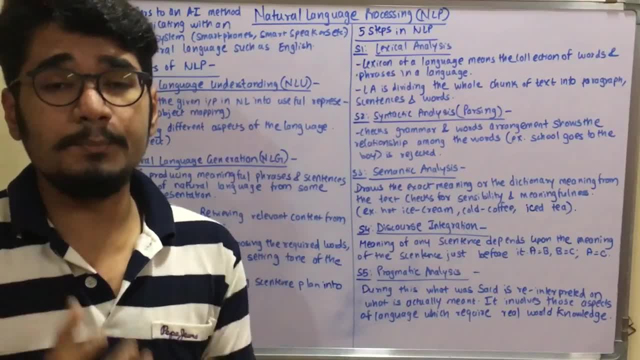 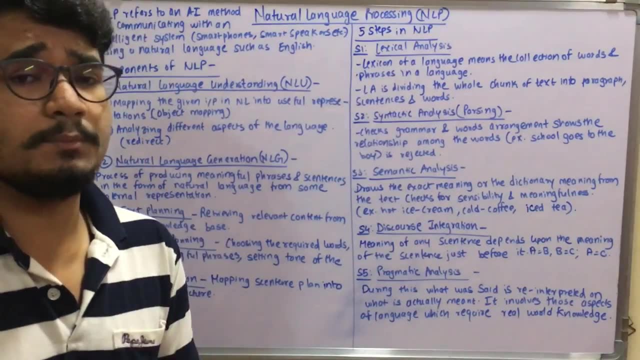 have the vocabulary of that many items so that i can reproduce them into my sentences or i can formulate in a very constructive manner, so that understanding is very much important in each of the domain. it's not about languages, but then also when you learn all the technical subjects and all 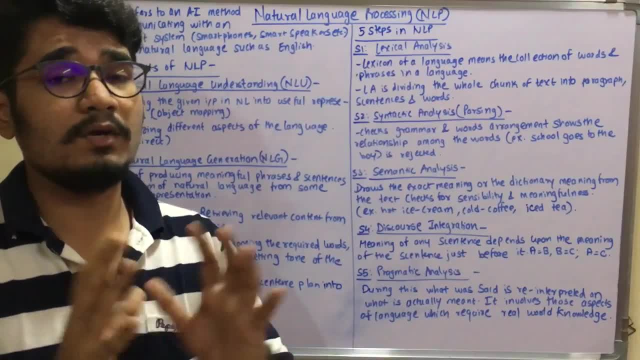 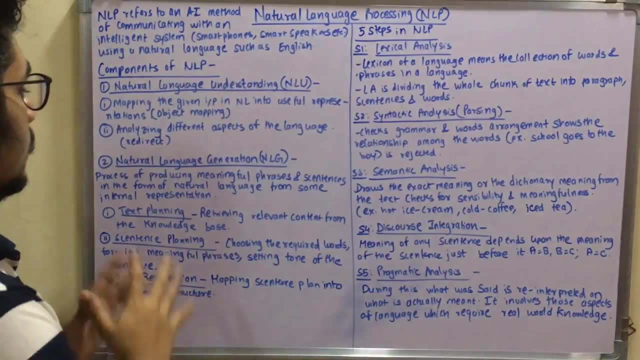 the real world things you have to first understand. if you don't understand, you cannot generate it. so it's simple as that. so the second step in nlu is analyzing the different aspects of the language. so it's like a direction to that particular point now, like particular object. 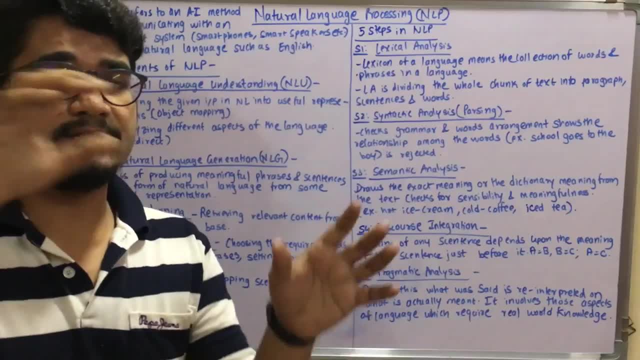 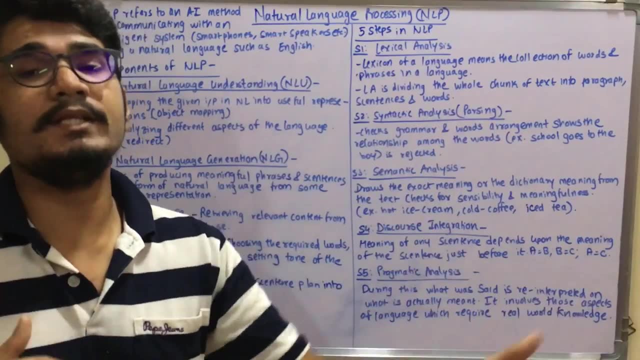 apple is there or a ball is there. so in what context? all these objects are being directed to one particular point. so that thing is very important. means you have to direct or you have to relate and study those things. so that is the important thing in nlu, that is the natural language understanding. so once 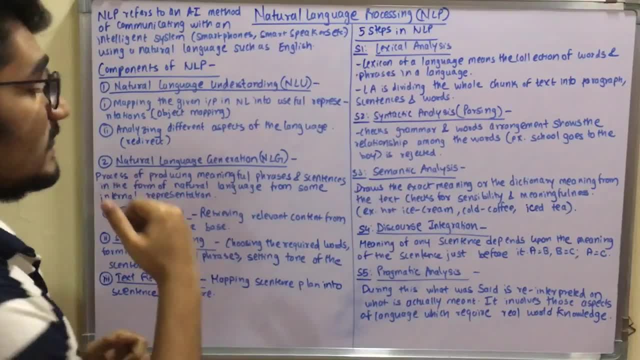 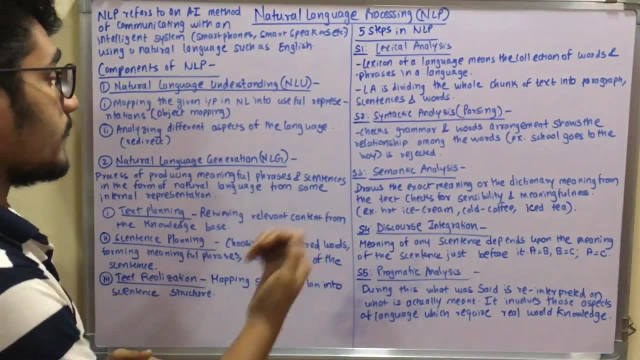 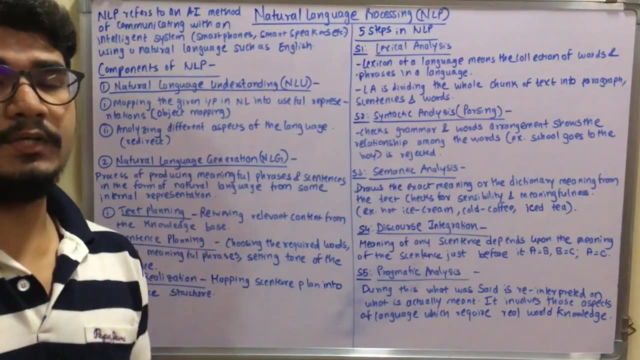 if you have understood what is natural language, then you will generate by your own, like natural language generation energy. so it is the process of producing meaningful phrases and sentences in the form of natural language from some internal kind of representations means, for example, say, tomorrow we are given an assignment of doing a college presentation, or kind of 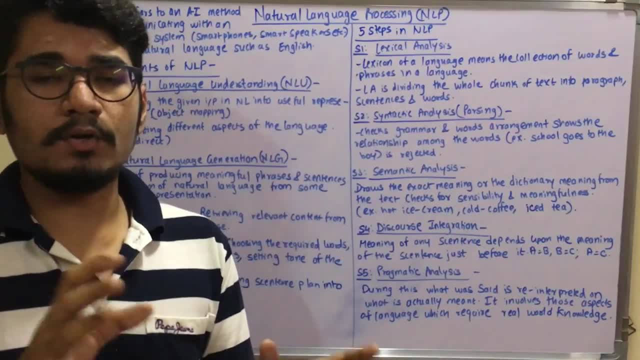 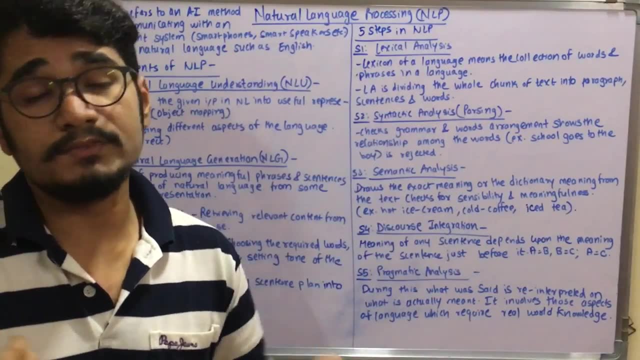 seminar is there. so what do you do? you go on Google, you search for that particular topic. what do you do? you extract some kind of paragraphs, you analyze some sentences, you make some your vocabulary- you will have your kind of own vocabulary- and then you try to jot it down on a paper and then you prepare. 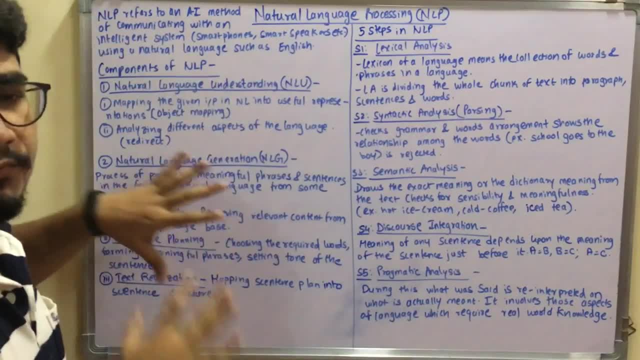 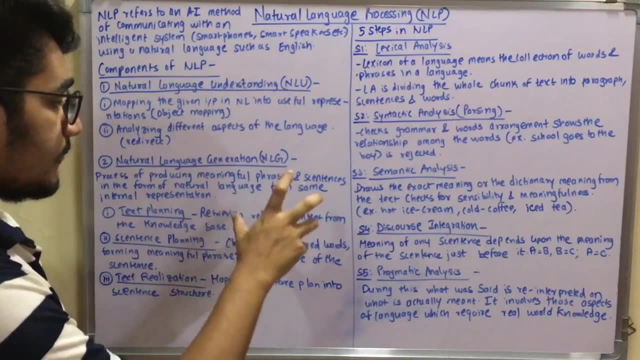 yourself and then you give it your presentation. so it works in the similar fashion. so you have three steps in that. so first is the text planning, so it is basically the retrieval of relevant content from the knowledge base. you have your own vocabulary, but then to check whether that vocabulary will be able to provide a good work experience rather than the kind 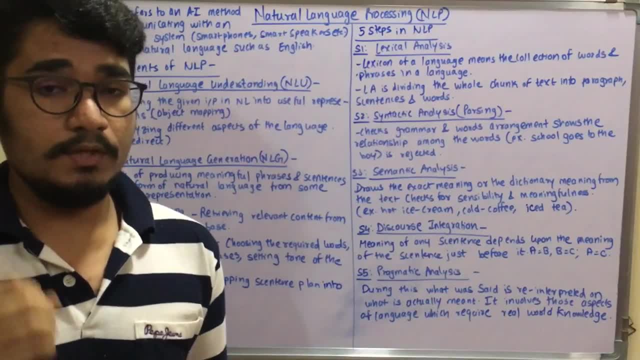 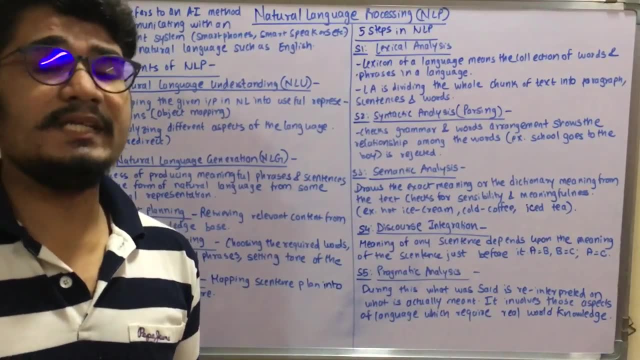 vocabulary is right to your situation, then you have to review it, you have to retry or you have to double check it what its real meaning is. so you need to actually plan those text. so in each and every step planning is very much important. so in life also, if there is no planning you cannot do. 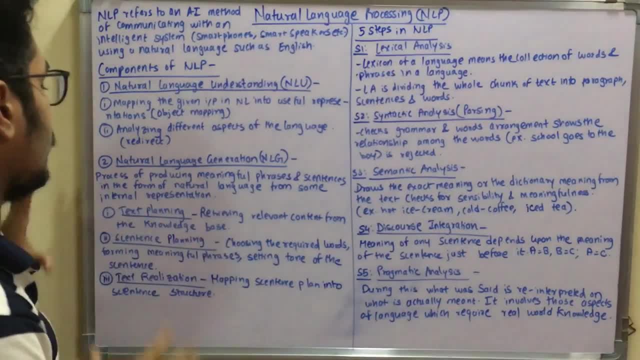 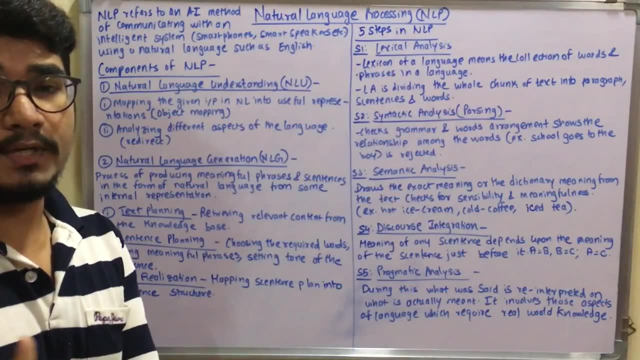 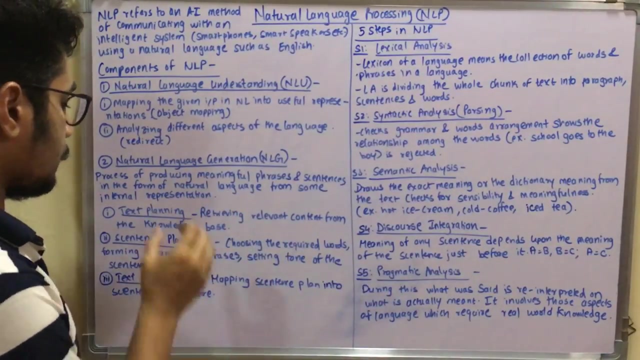 anything in life. so it goes with the same in case of nlp as well. then you have the sentence planning. once you have the appropriate text for your particular kind of command or particular kind of system, then you have to framework that particular sentence, so choosing the required words, forming 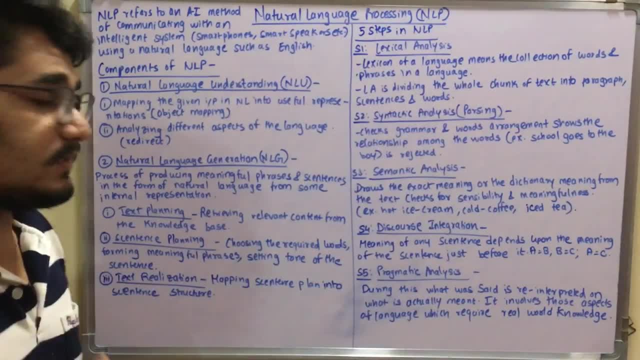 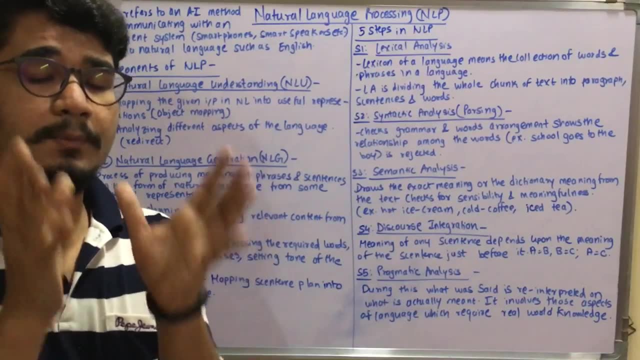 meaningful phrases and setting the tone of the sentence. so that's very important. like you have to choose those particular sentences and form one particular grammar and it should totally make sense to your command. like, for example, if you have your amazon, alexa and you are saying, hey, alexa. 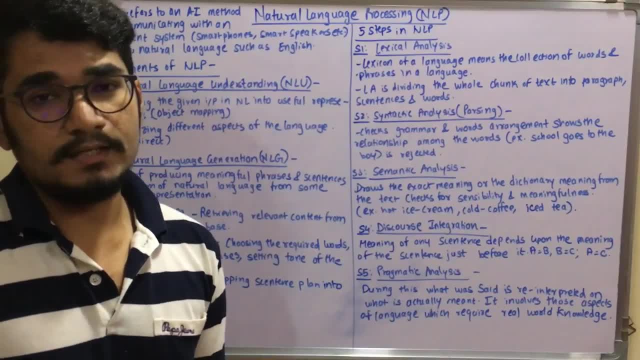 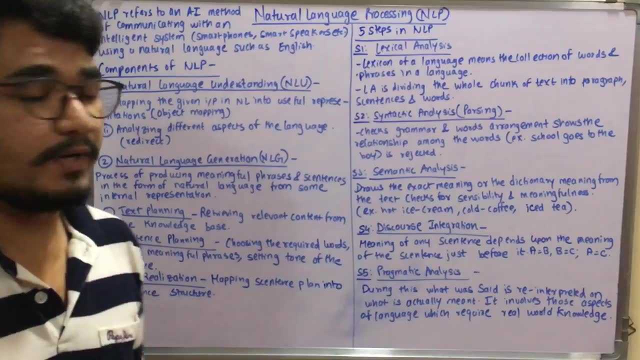 then it will not listen. instead, alexa, then it will listen. so that kind of tone differentiation should be there. so that's the first thing you have to do. so if you have a system like that should be there while you do the sentence flying, so that's very much important. then you have the 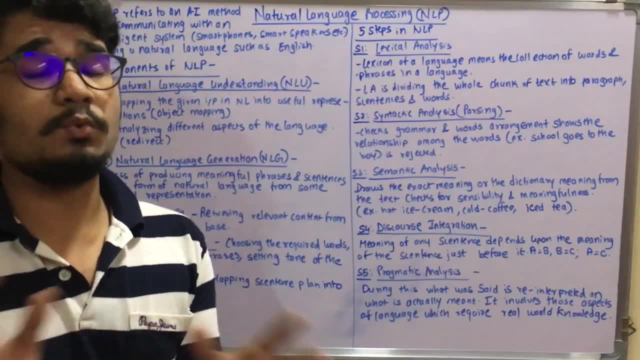 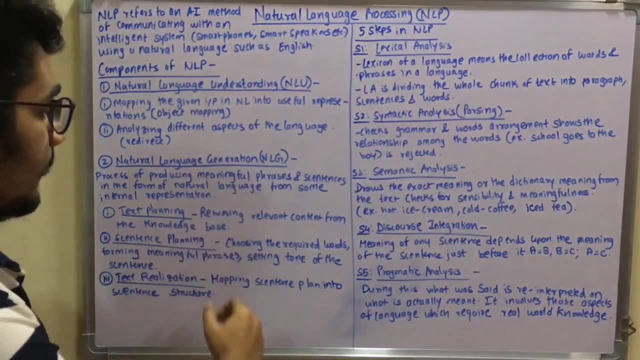 text. realization means you have to realize whatever you have written is true to your knowledge, so that's very much important. and then you will give your presentation to the end user, so you have to realize that mapping each of the sentence plan into sentence structure, so that's very much important. 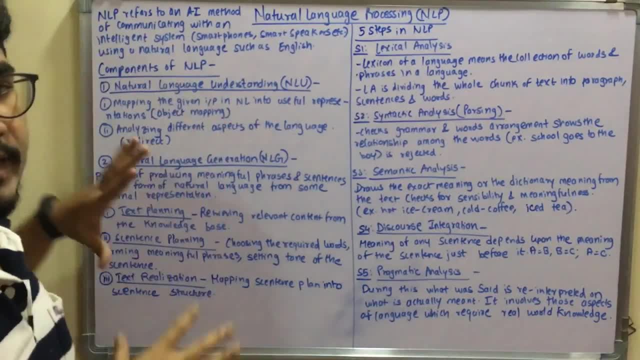 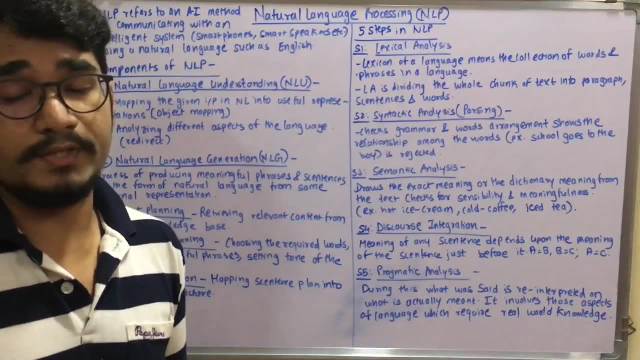 in natural language generation. so we have seen the components of nlp, that is, natural language understanding. first you have to understand that language and then you have to generate that language in your particular way. so everyone has a different way of producing their own language. so that's. 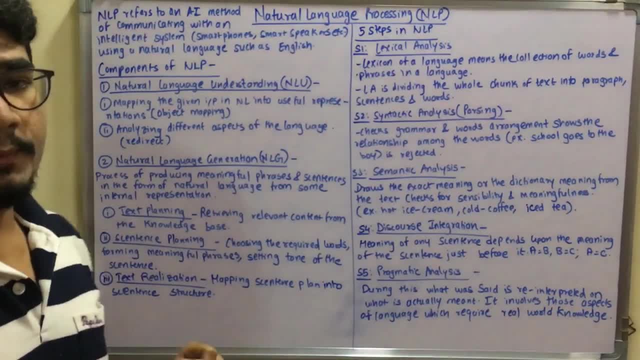 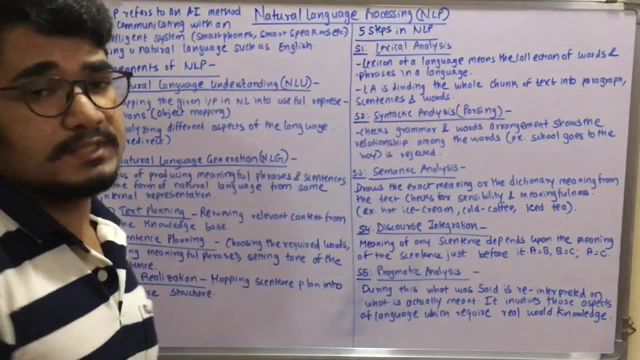 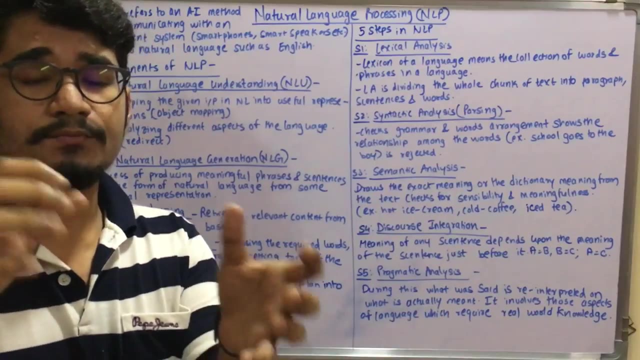 difficult from uh individual to individual. next we talk about these steps. so there are five different steps of natural language uh processing, so how this processing takes place. so the very first is lexical analysis: what is lexical or what is lexicon? lexicon is nothing but words or vocabularies, for 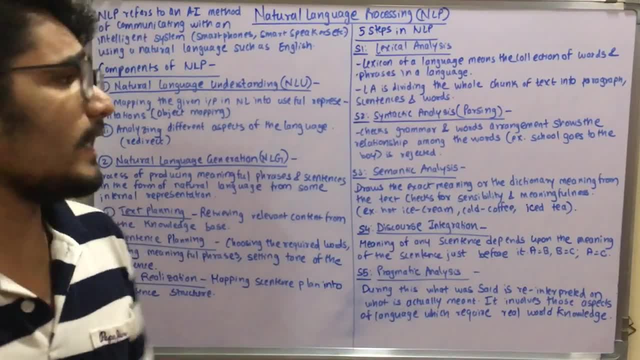 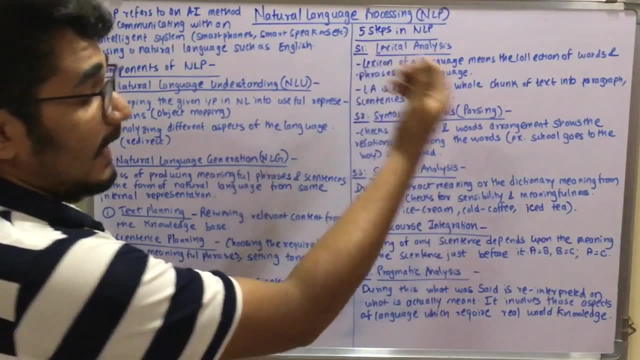 that particular language. it may be kind of jargons or many kind of things. so lexicon of a language means the collection of a language, and then it is the collection of a language and then it is the collection of different words and phrases in a language. then uh la is divided that this lexical. 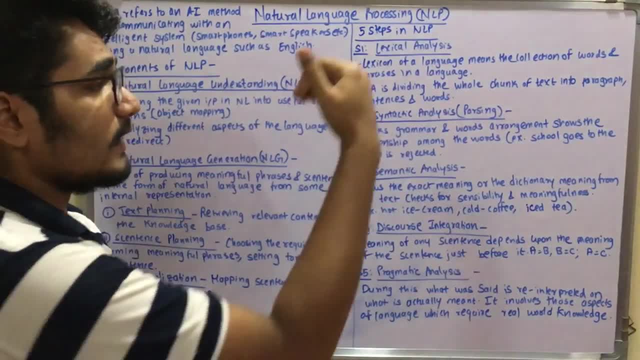 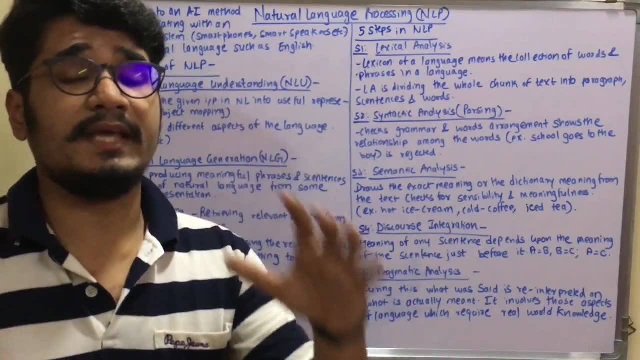 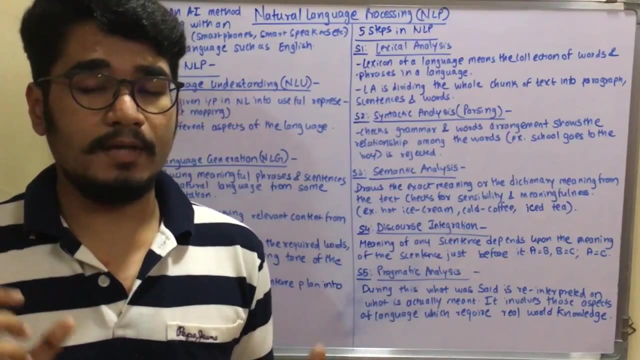 analysis is uh being dividing the whole of chunk into different paragraph sentences and words. like you, have many uh apps, and all in android, so what it does is basically scans one particular entire paragraph and then it tries to understand what is it particular sentences, what that word actually. 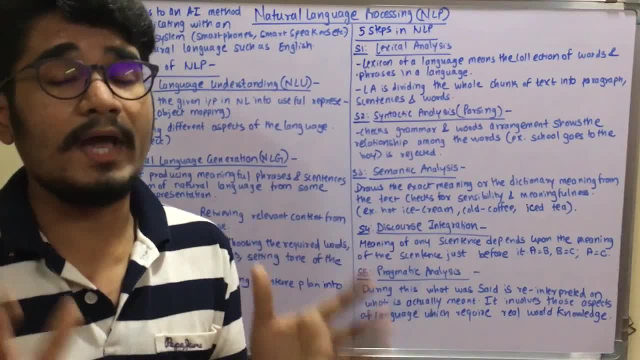 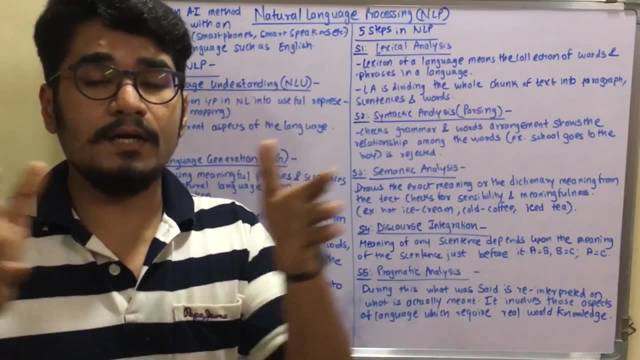 means. so it's like a kind of natural language processing. so first you need to have that particular knowledge base, that is lexicon analysis. each and every word, each and every alphabets, so from alphabets it uh joins the words, and from joints you frame sentences, and from sentences you frame paragraphs, so that becomes. 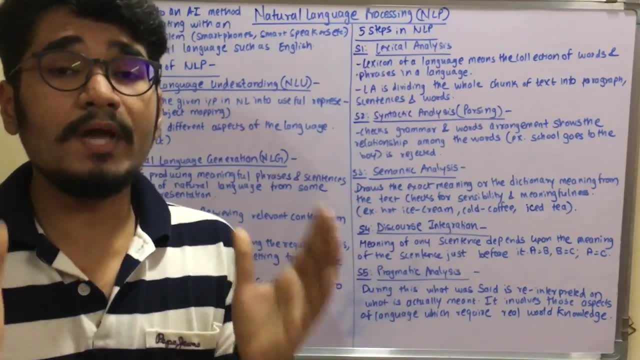 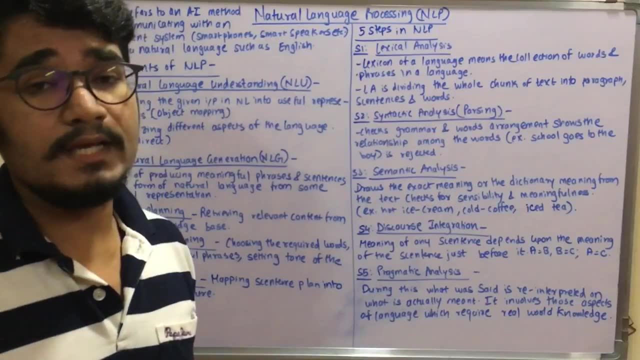 the story, so it's like a big picture and all together. so you need to have the first, that is, lexical analysis in that. so that's very much important once that is done. then you have the syntactical analysis, that is, parsing. we have different, different coding languages. uh, we have. 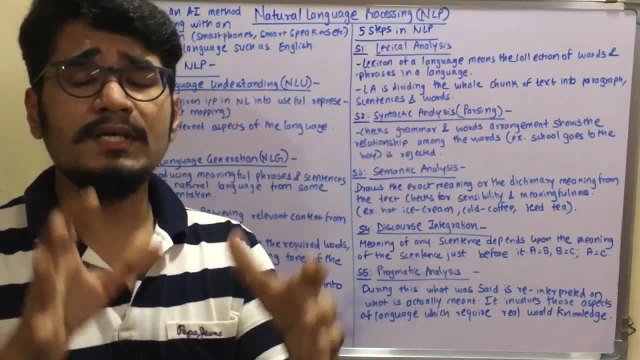 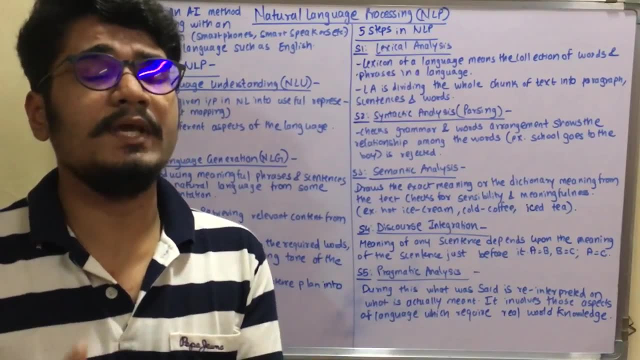 java, python, c, sharp r and all these things. so this has got its own certain kind of compiler sets it has. so what it basically checks is it basically checks at the run time whether those particular commands which you gave are the syntax, whether it is correct or not. so it 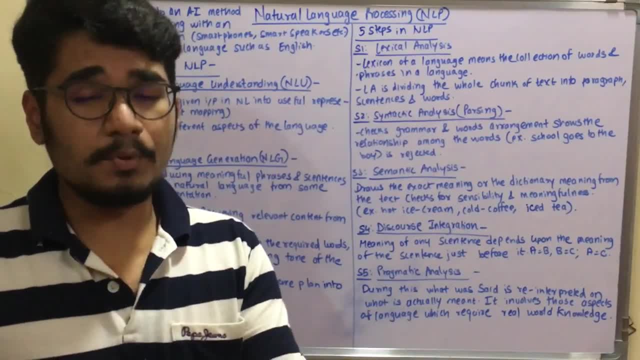 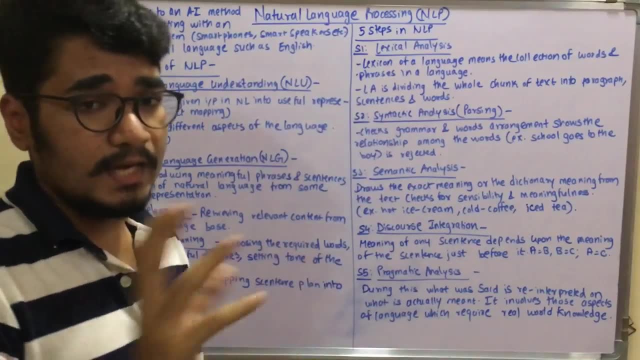 basically checks for the uh grammars and all those things, whether it's written properly or whether the semicolon or where the brackets is given properly and all. so it basically checks for that. so similarly in nlp also it goes in that way. so syntactical analysis, that is, parsing, is very much. 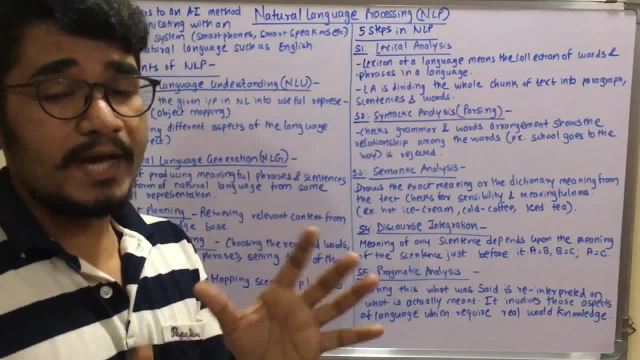 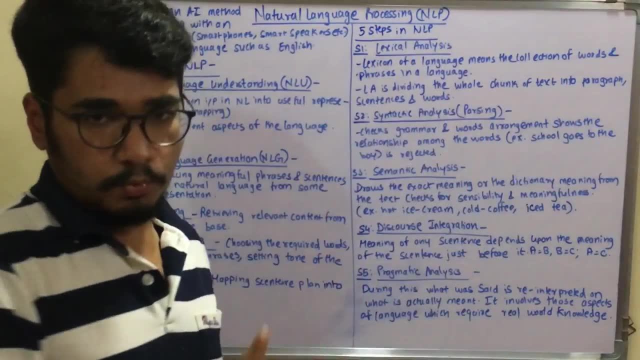 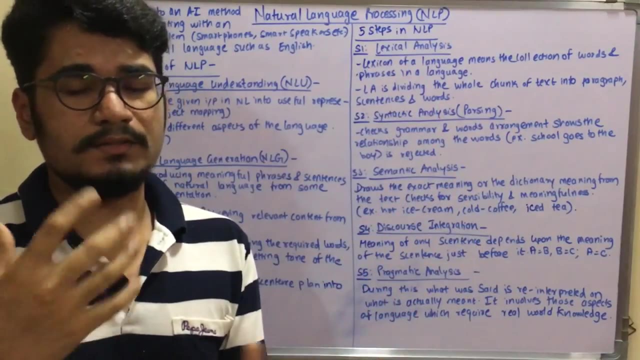 required. it checks for the grammars and the arrangement of the words or the fashion of words, the relationship among different words, like, for example, if i say the school goes to the boy, in the real world it doesn't makes any sense. like, uh, school is what, it's a non-object or it's a 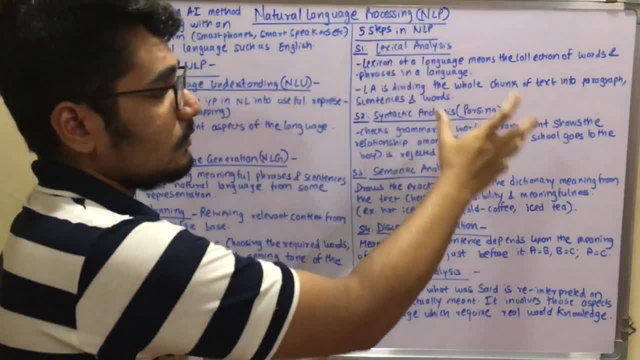 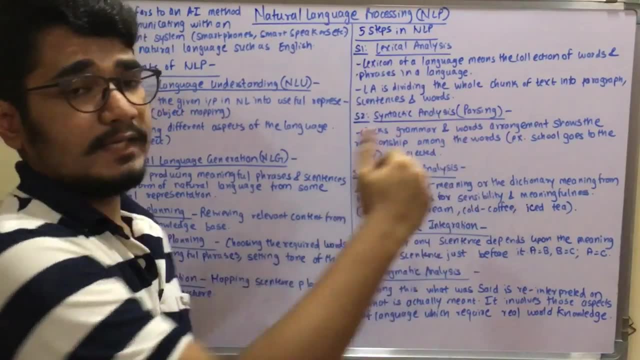 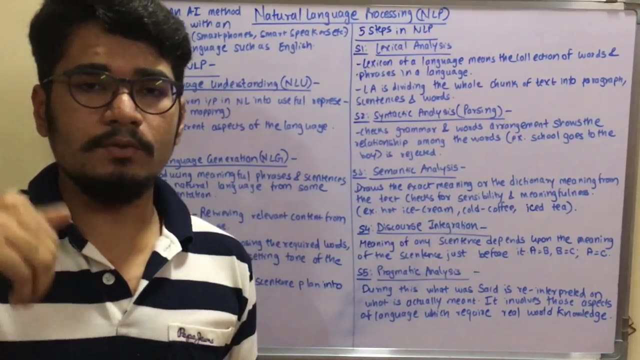 non-living thing and boy is a living thing, and though school is a static object, uh, then it goes to the boy, then it's uh like uh rejected. if it's like the boy goes to the school, then that uh makes a sense like a boy is a uh, what you can say. it's a living object, so it goes to. 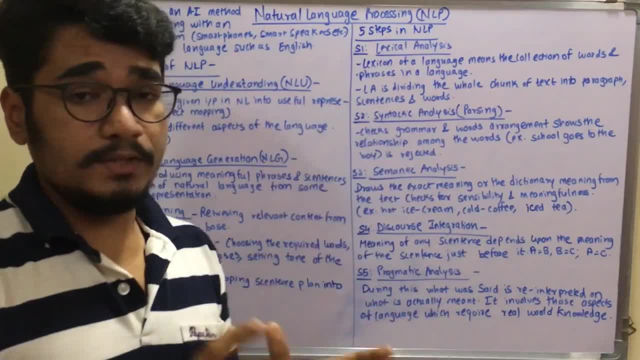 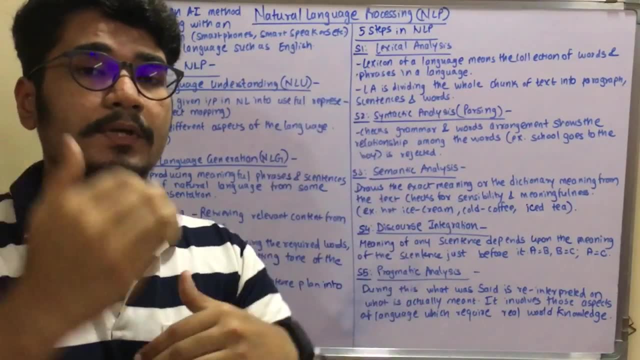 a particular kind of uh building, so it, the nlp or the machine, has to understand that school is a non-living object, it is a static object, it is made of bricks and all these things, so people go into that building and also that thing or that information or that level, kind of. 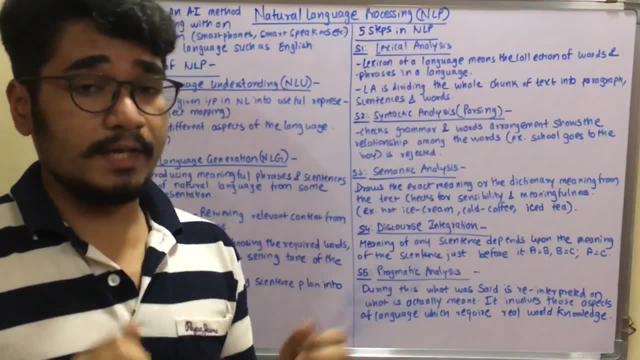 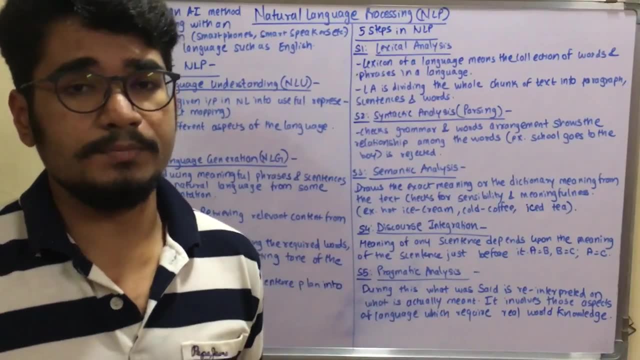 categorical hierarchy that you must very much incorporate into your ai system. so that's very much important. and so if i say a drone goes to the boy, this makes sense. like drone is also non-living object, but it has its own kind of specifications and all. so it's a that's a non-living object. so we. 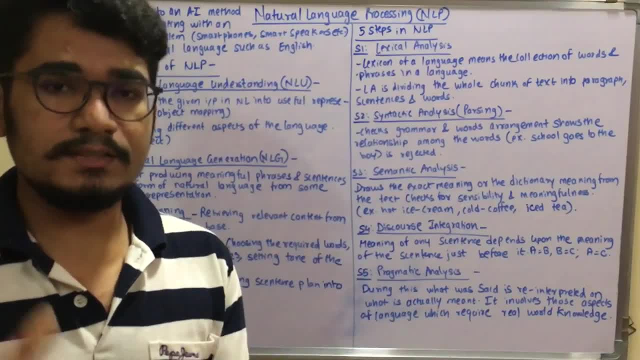 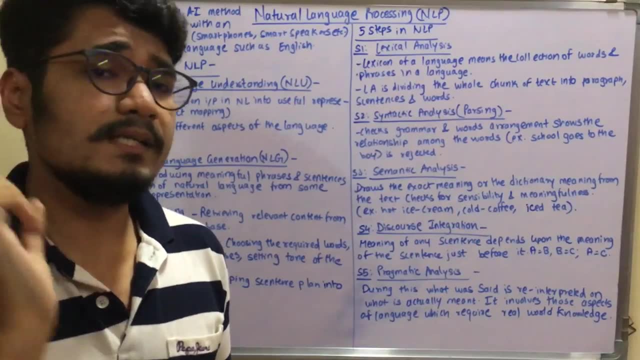 like. we have to understand that concept or whether it's called. So that's mainly important in this. then you have the semantic analysis. semantic is nothing but the meaning, so we have to understand the meaning of that particular sentence, what it's actually trying to mean. 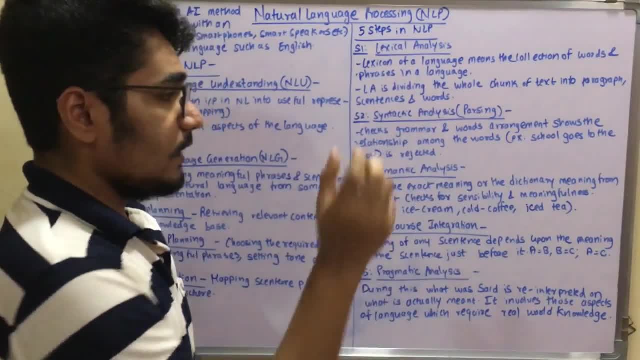 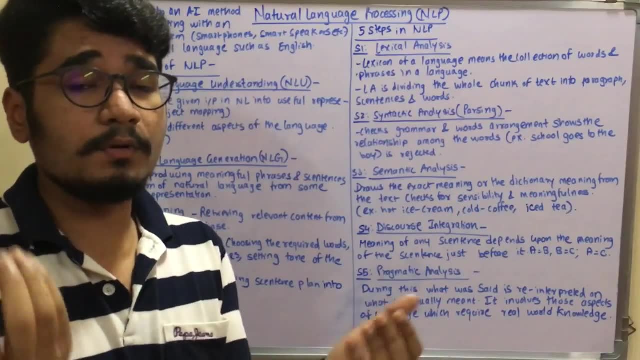 So it draws the exact meaning or the dictionary meaning from the text and checks for its sensibility and meaningfulness. So whether checks whether it's sensible or not sensible for me to understand or sensible for me to produce it to the end user. so it well, very well, checks for that example. 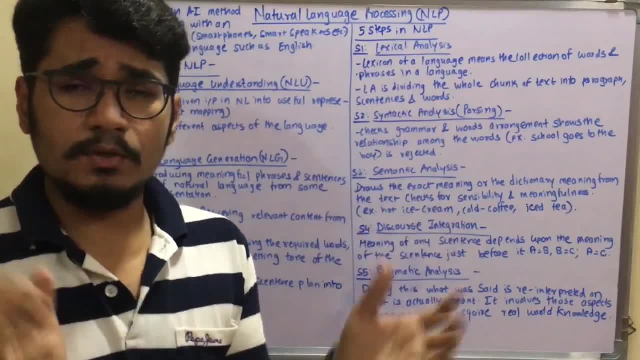 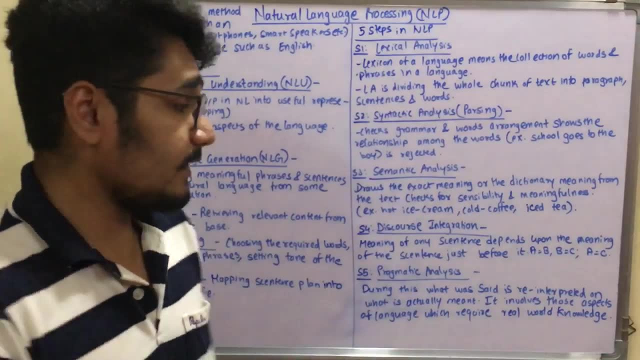 If I say hot ice cream, so what does ice cream? basically it's a very cold object. you it's a delicacy that you have like as a desert, and also it cannot be hot, Whereas if I say cold coffee, coffee is hot, but then you can. 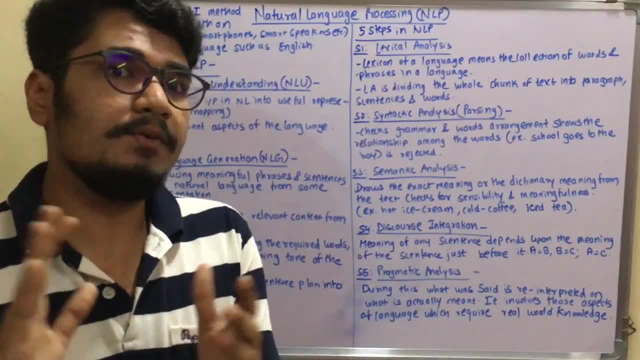 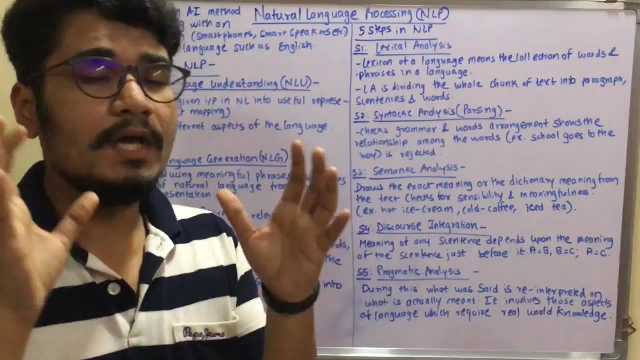 have cold coffee with iced and all those things. So it's like in a different context you have to identify what it actually means, or in the real world, if these particular things are there or not, so that you have to very much have a sound knowledge. 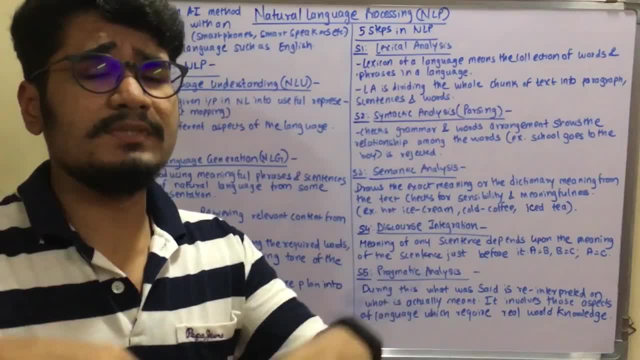 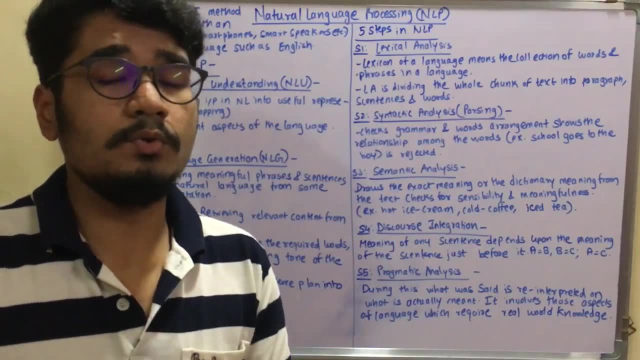 For that. then you have iced tea. tea is also hot, but who puts ice in that? but then to iced tea. a kind of thing is there. so that's very much has to be understood by the machine, Although you know, but machine doesn't know, so you have to. 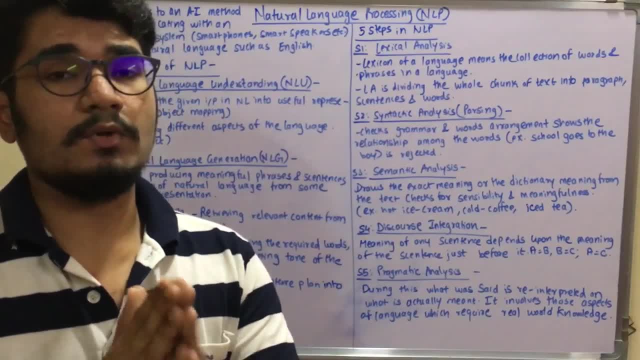 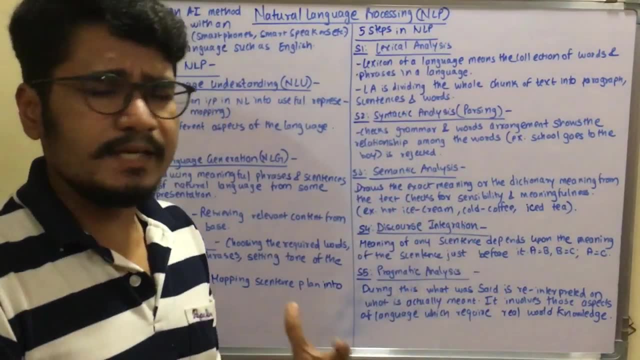 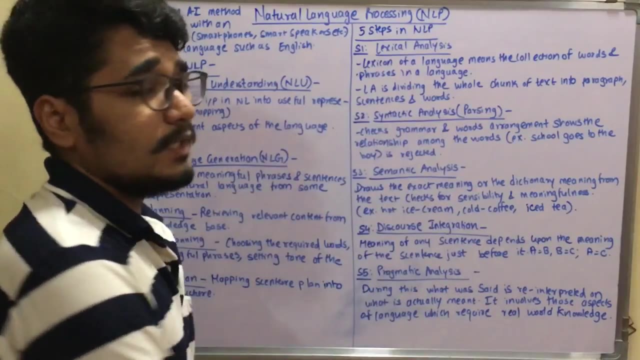 teach that machine. so that comes in machine learning, So how machine learns all these things. then comes the disclosure, integration. So it's nothing. but the meaning of any sentence depends upon the meaning of the previous sentence just before it or the precursor to it, For example. 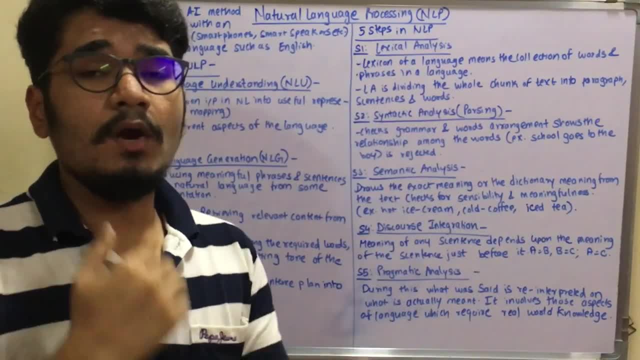 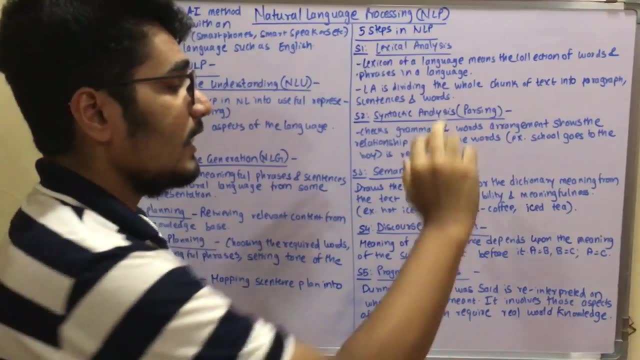 If you have a sentence, like in mathematics of the relation, a is equal to B or B is equal to C, So what you does, if you like, have, a is equal to C. So it's like if a is equal to B, B is equal to C, then a is also. 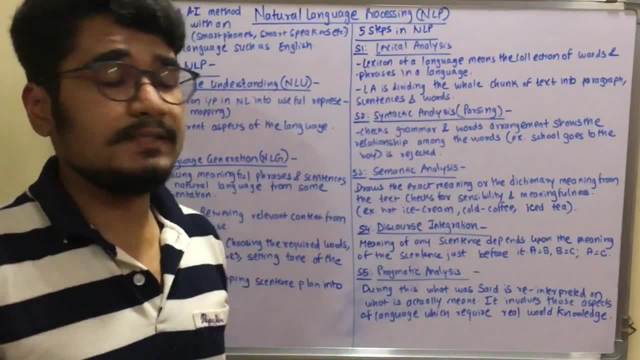 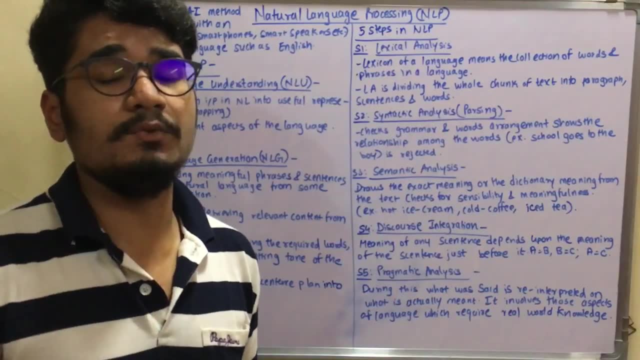 equal to C. So it's in that way. Then you have the pragmatic analysis. pragmatic in real world is nothing but practical. You have to practically analyze those things, whether which is said by the user It's practical or not. So for that, during this, what was said in the reinterpreted and 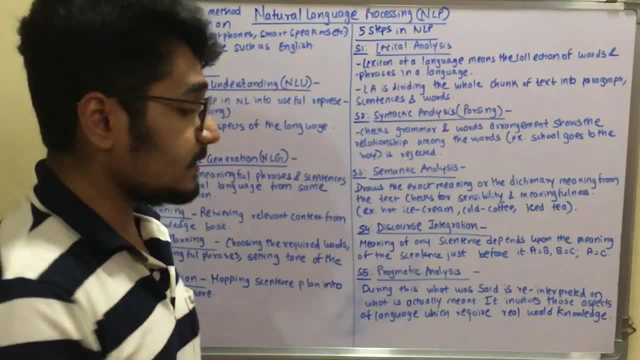 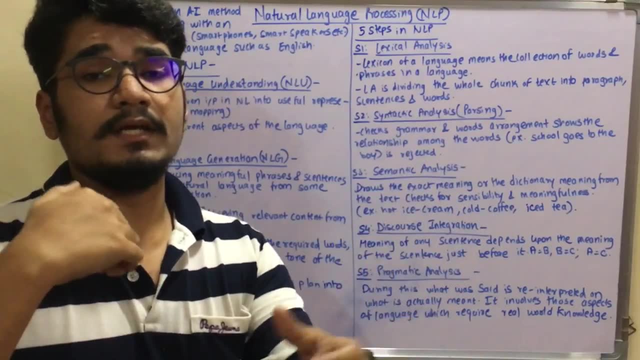 what is actually meant. So it involves those aspects of a language which require real world knowledge. So what a user tells to Siri: Siri, hey, Siri, how's the weather today. or Siri, find me some restaurants to nearby. or Siri, check my mails. and also it should make some kind of thing. 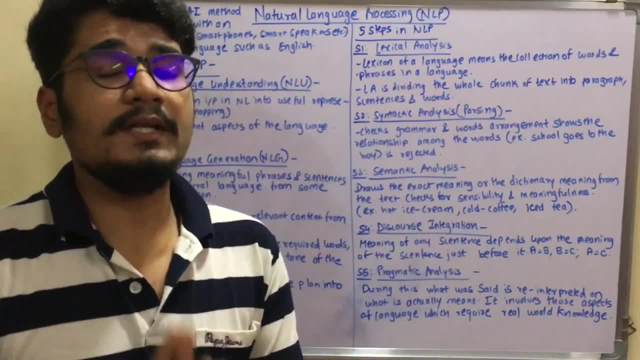 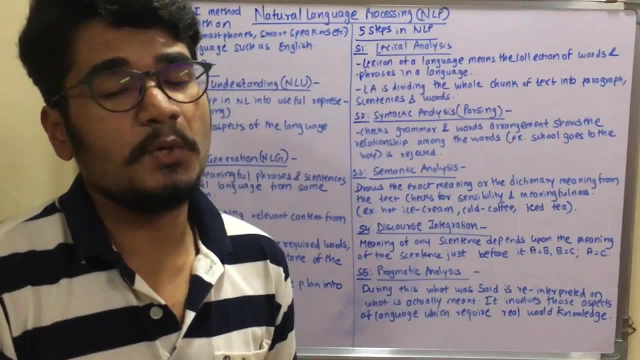 so that the system should also respond in that way. So well, that was all about regarding the natural language processing and artificial intelligence, So hope you guys enjoyed this video. Thank you for watching this video. Please do like, share, comment and, most importantly, don't forget. to subscribe to my channel. Thank you very much.